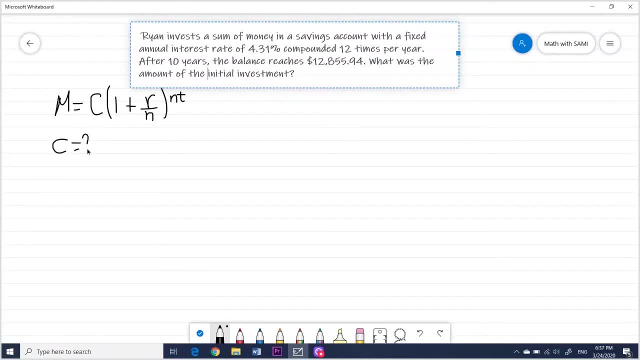 now that we need to find the investment. so the final amount, because it says after, after ten years, the balance reaches twelve. so M equal to the final amount, twelve thousand eight hundred fifty five point ninety four. the rate is four point thirty one percent, and always that I have to divide it by 100 is 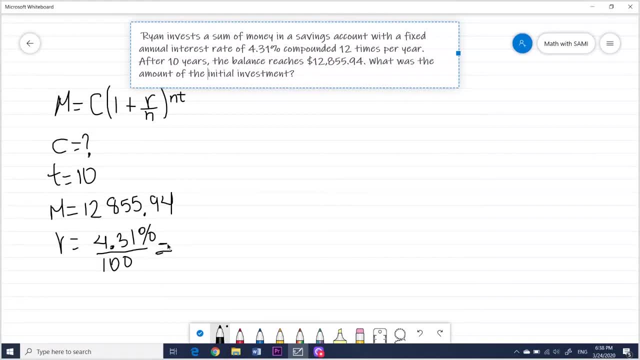 going to be equal to. you have to use your calculator if you don't know how to do it. zero point zero, four, three one, n is equal to 12. remember that the period represents the amount of times that the interest is going to be compound per year. 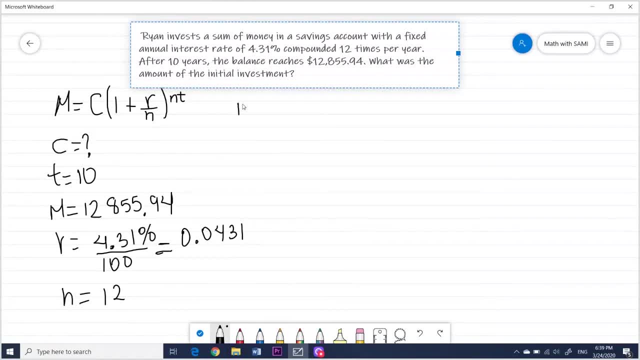 okay, So M is going to be equal to 12,855.94. equal to C multiplied by 1, plus rate equal to 0.0431 over N. N is 12,. elevated to the power of N is equal to 12 multiplied by T. 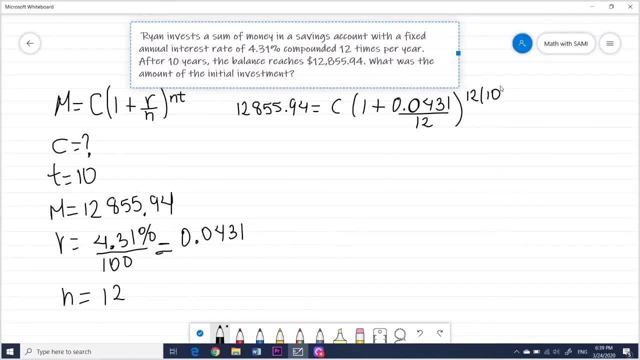 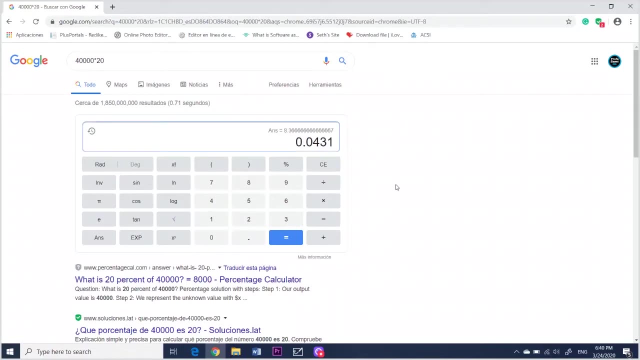 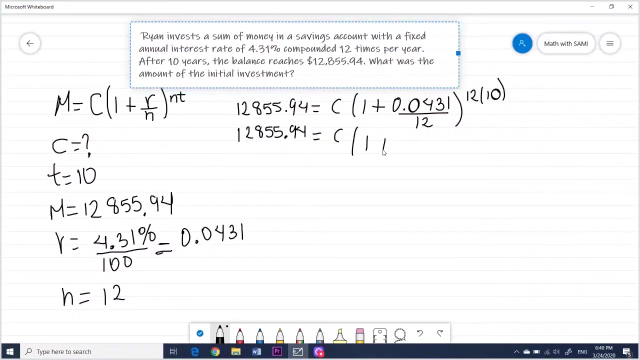 T is 10, okay, So now I'm going to do everything inside the parentheses. I'm writing down this again: C. so dividing that 0.0431 over 12. 12, 0.0036,, 1 plus 0.0036.. 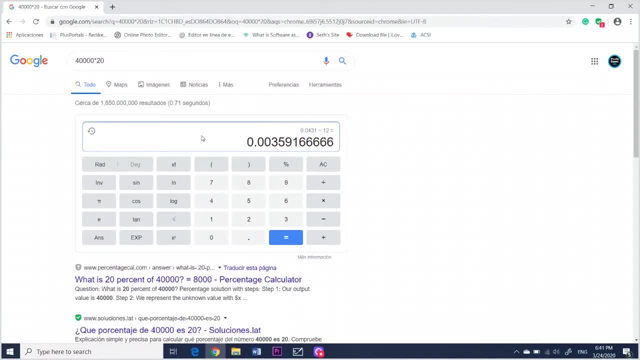 Okay. the reason why I'm choosing four digits after the decimal in the decimal place is because if I select only two, I'm going to have a zero, So I need to select at least four in this case. okay, But it's okay if, most of the time, you select just two digits. okay.